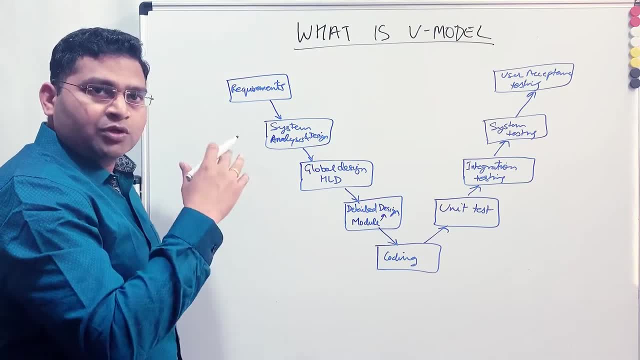 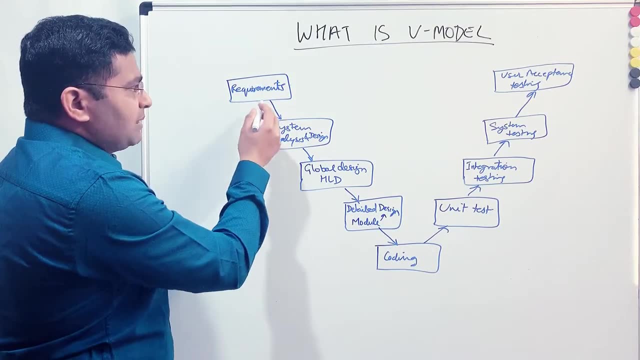 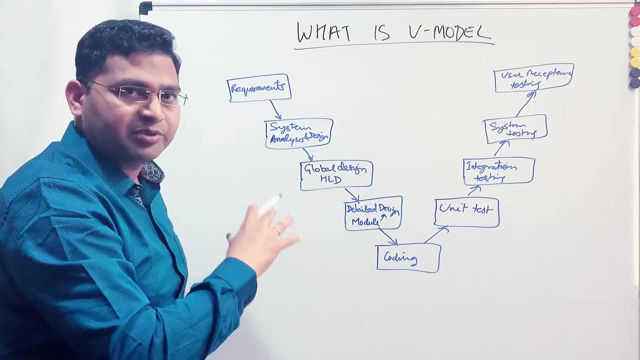 development team to start working on any of the coding or development activity. So once the requirements are available, so requirement gathering. So in that particular phase, in the software, in the waterfall approach, there was no test involvement at that particular phase. So once the requirements got frozen, only then the development activity or the 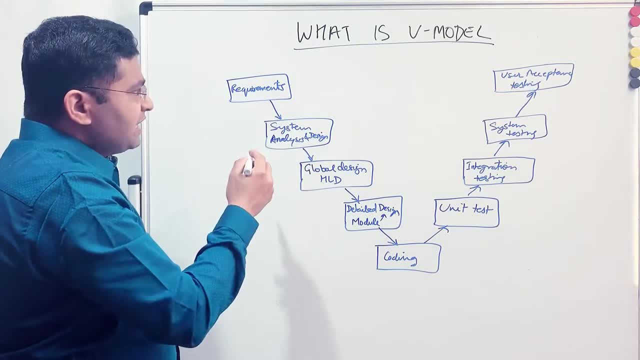 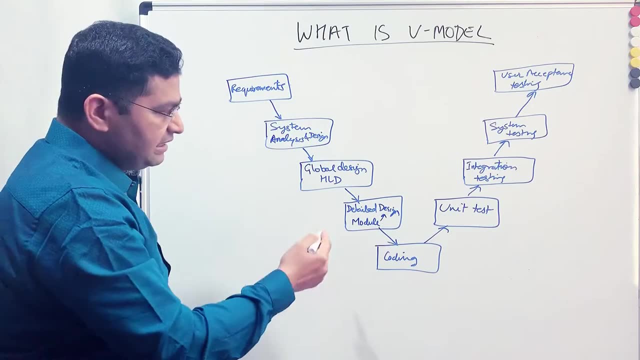 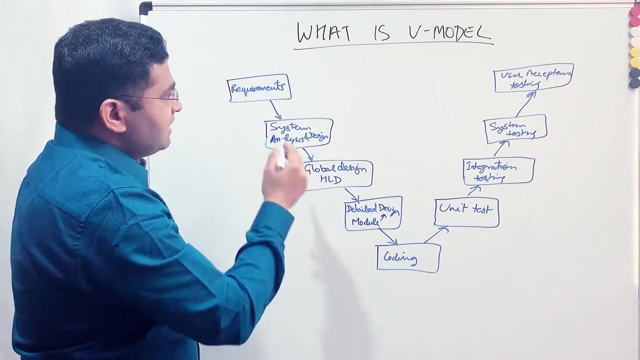 design activity started in the waterfall approach. Now, because of that, the defects that could have been found in the requirement phase itself were delayed until testing or the deployment happened To overcome. that vModel was introduced And in this, if you see, there is a corresponding involvement. 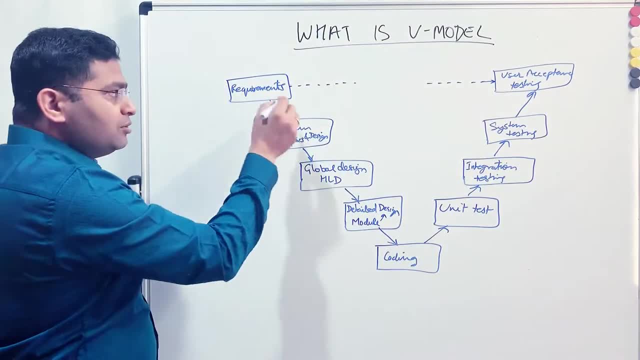 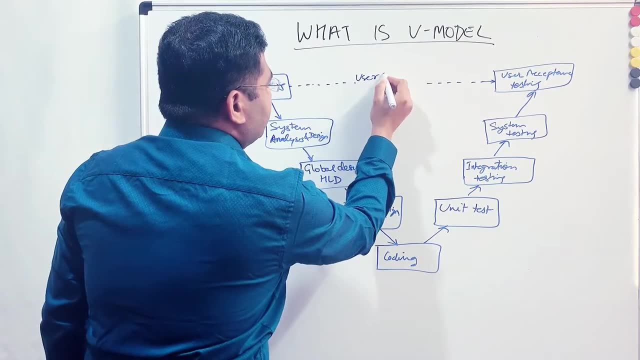 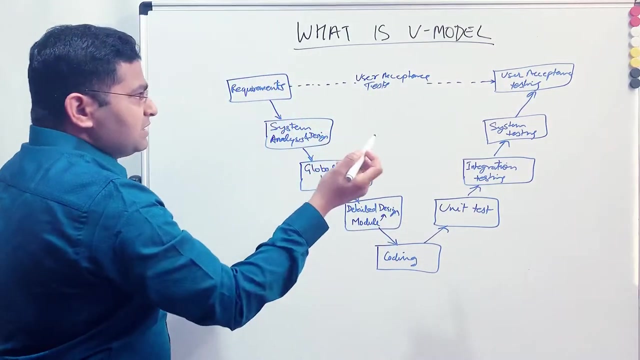 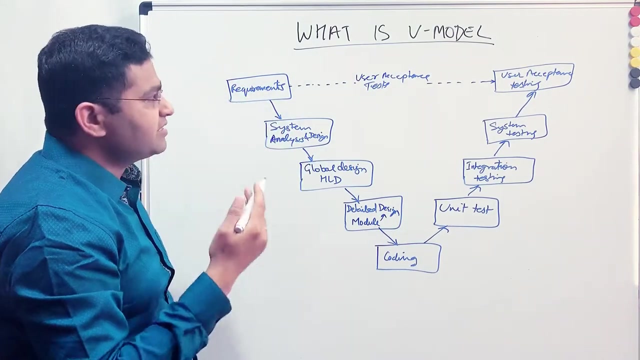 of test team. So as soon as the requirements are available, testing team starts writing the user acceptance tests. Okay, So what the testing team does is they go through the requirement and, based on those requirements, they start documenting their test cases. or basically, at this level they can understand. 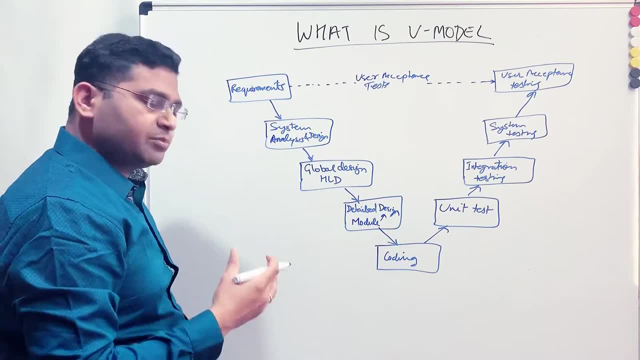 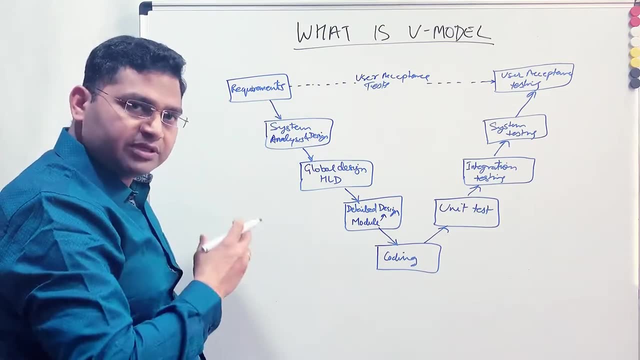 what the high level requirements are and, based on that, what customer is looking for. And when they understand those requirements, they go through those requirements. they are involved into the discussion with the team, with the customer. then they can write the user acceptance. 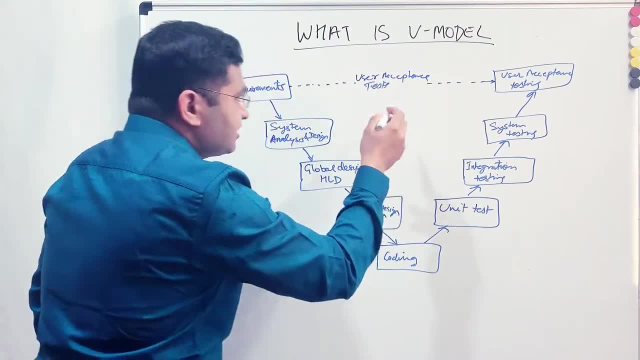 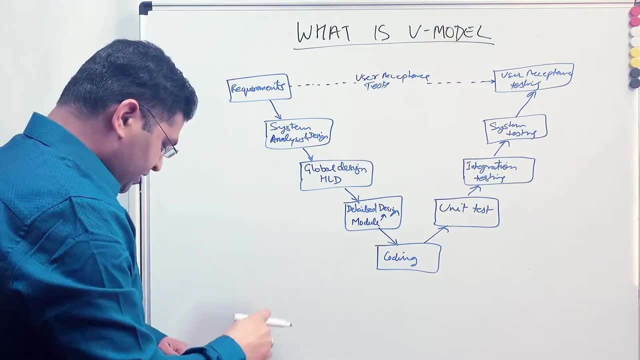 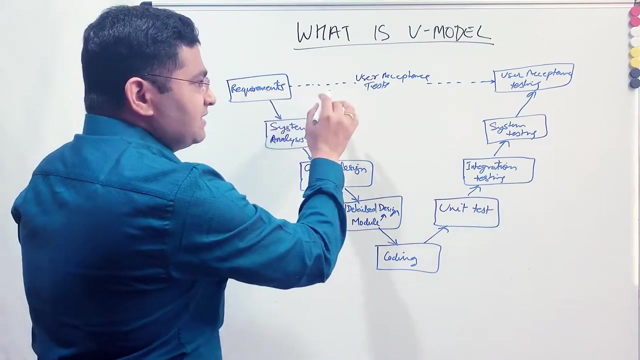 test cases. And when they are writing the test cases they come up with any of the gaps that might be there in the requirement gathering phase. So that's the first involvement, or the first within the first phase itself. the testing team is involved in writing the user acceptance test cases. 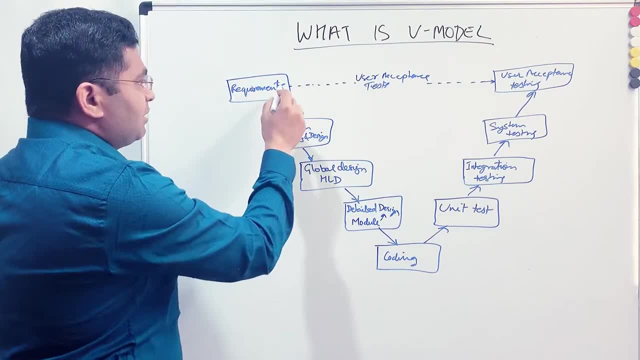 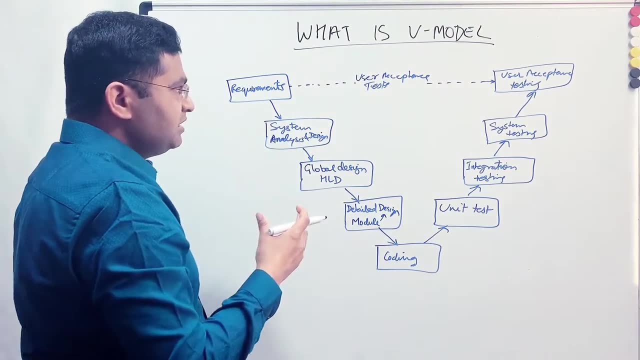 Now, once the requirements are being gathered and if you can see here after the requirement phase, then the system analysis and design starts. So when we say system analysis in the vModel, it's basically say, for example, you are developing. 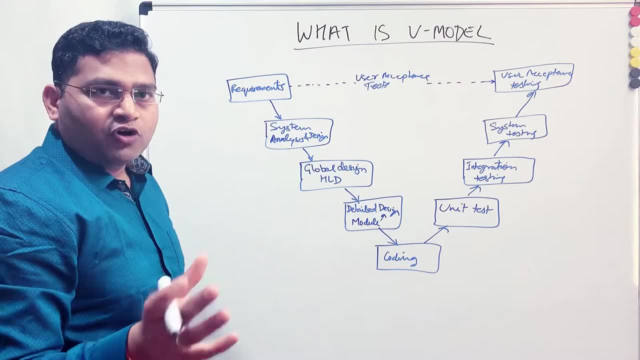 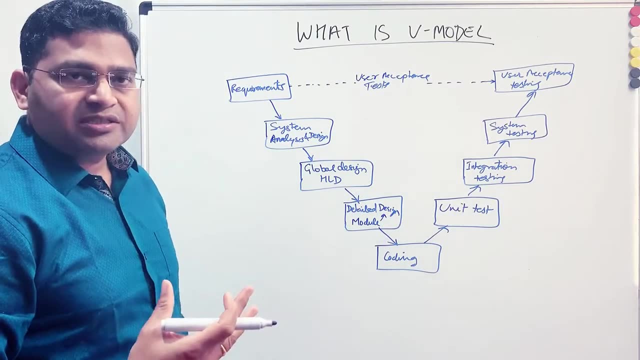 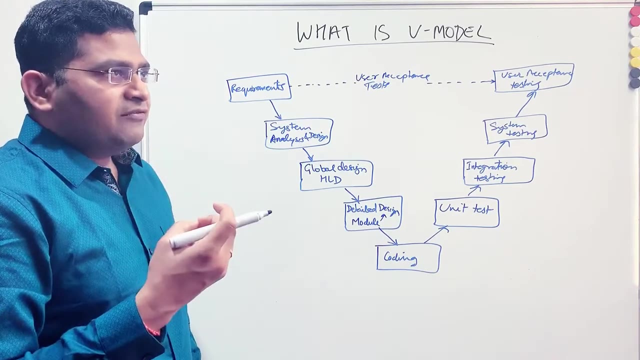 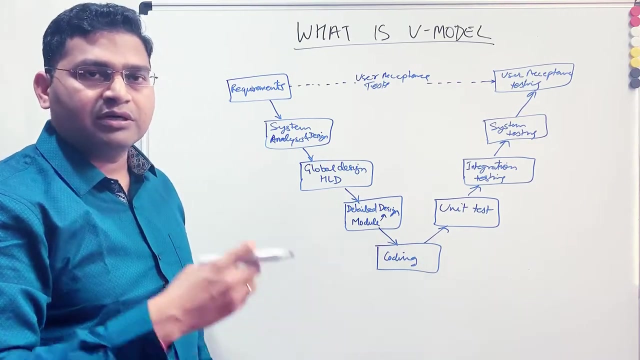 a banking application for distributing the cards, say, for example, right. So when you say the credit card or debit card, it involves the complete life cycle. There are different number of systems that are involved. So you will have a system to you know to originate the card, or a person or customer will come to originate or apply for the card right. 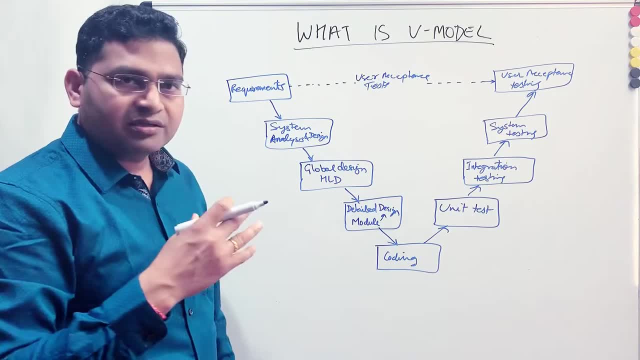 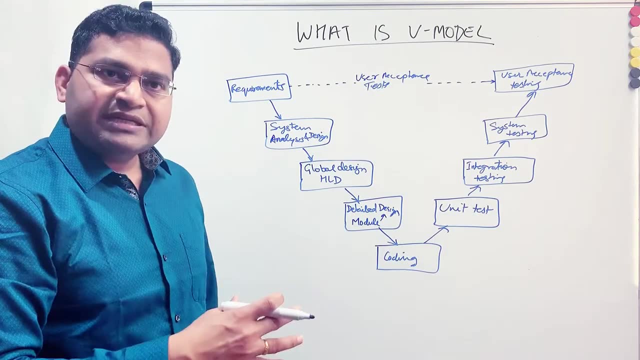 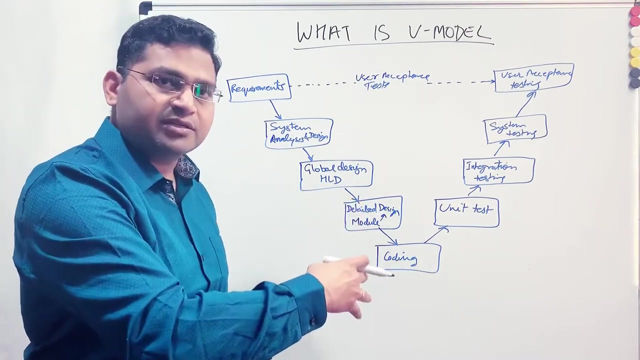 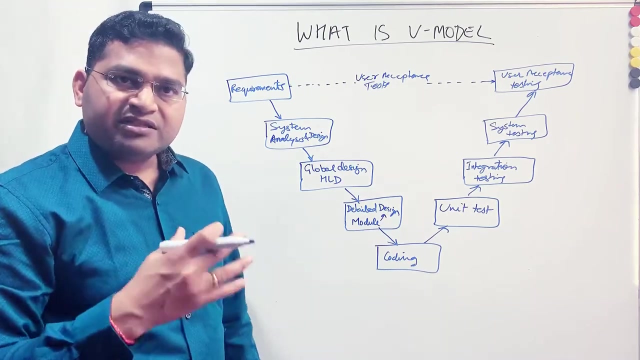 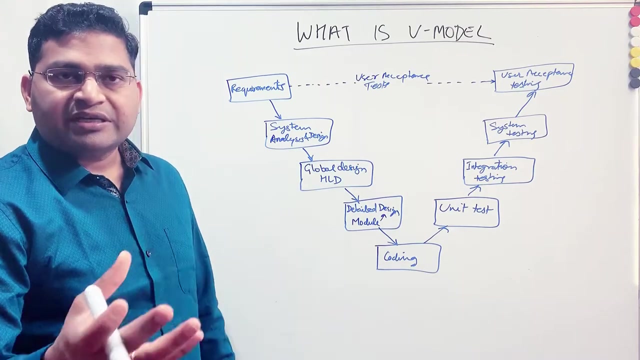 Once they apply for the card, then that card application goes into the backend system where there will be business process and the processing will happen. Once the processing has happened, then the card goes for embossing. So the physical card- right. So that goes to any third party or third system. So those systems are usually not maintained by the banks, right? So bank has the tie up with other system, other companies who do the card embossing or create the physical cards and send those. Similar is the case with the. you know all those letter generation and all 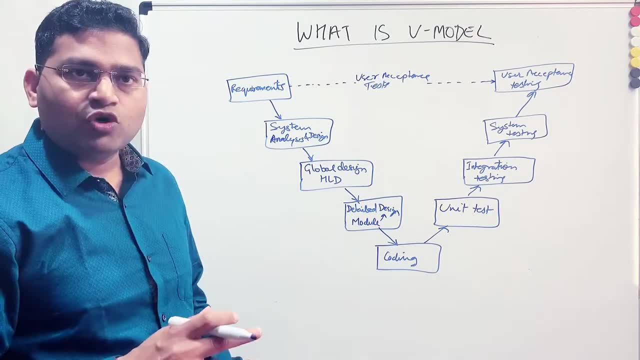 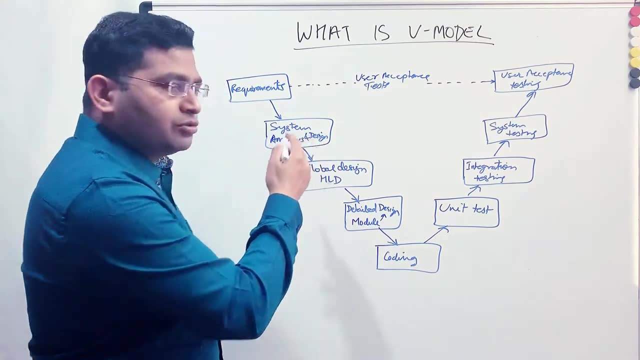 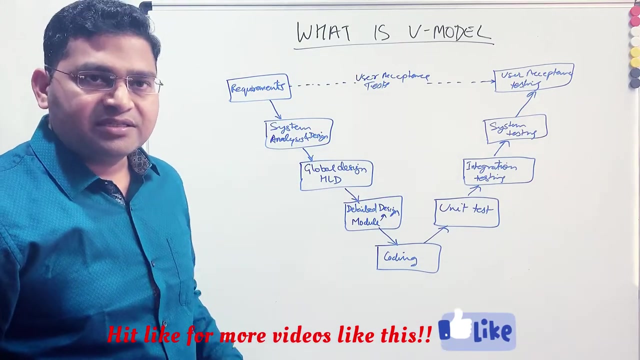 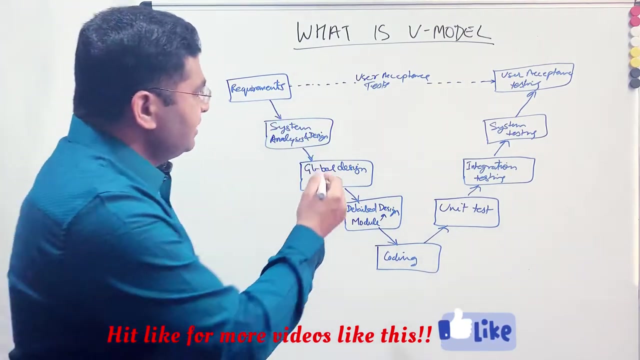 So if that is the case, there are different- you know companies involved and systems involved to produce the physical card, to produce the letters et cetera. then that understanding comes into the system analysis, So how that particular software will interact with other underlying system. that happens in the system analysis and design And once that system analysis is in progress, testers can at the same time write their system analysis. 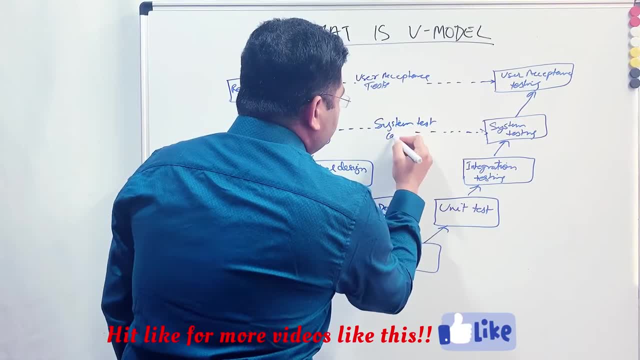 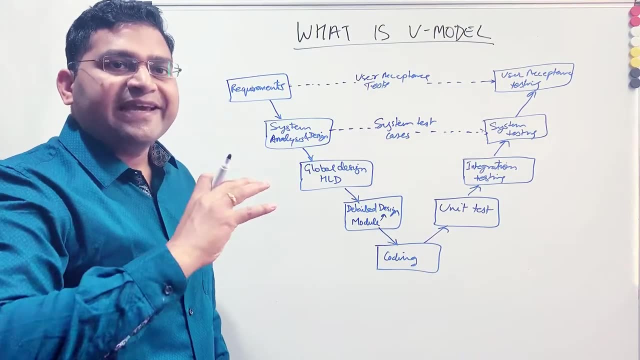 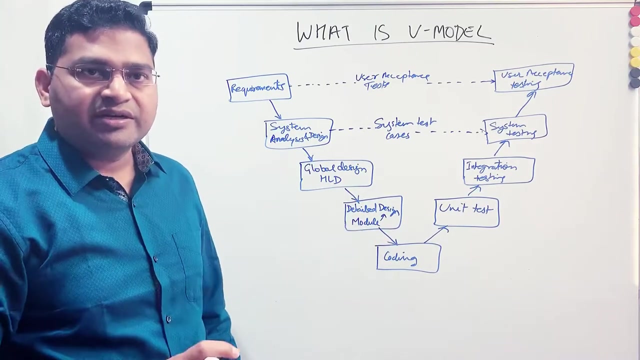 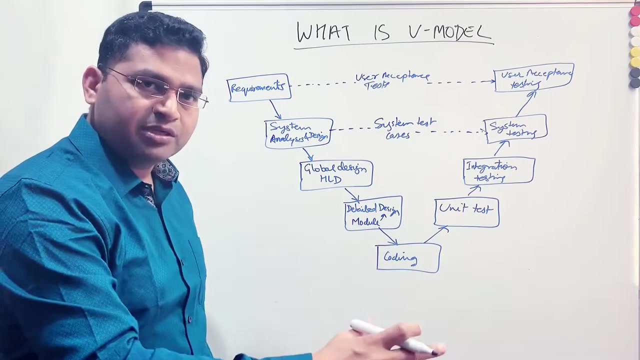 So what system test cases will do? is they will test or those test cases will target the end to end system? right, So they'll target when all the systems, different systems, third party systems- are integrated and how the overall testing will be performed in the end to end integrated system, be it, you know, like third party system or internal other systems that are, you know, available or involved in that particular system. 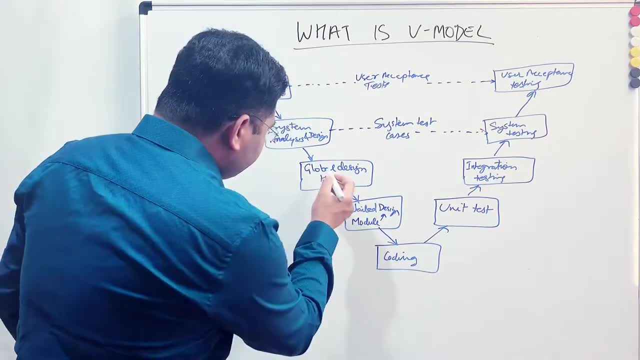 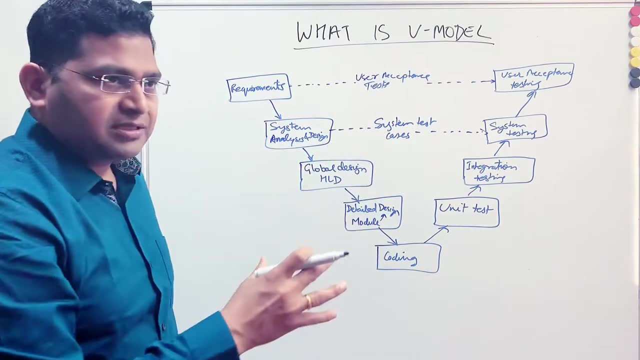 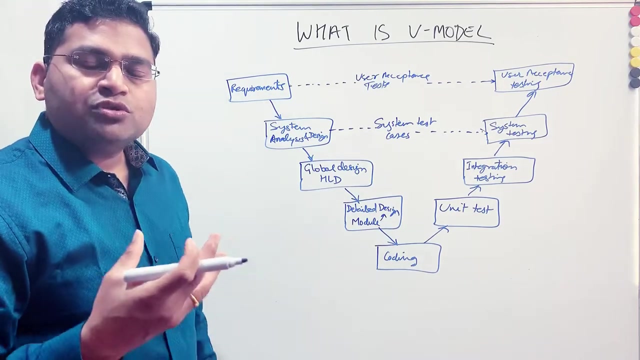 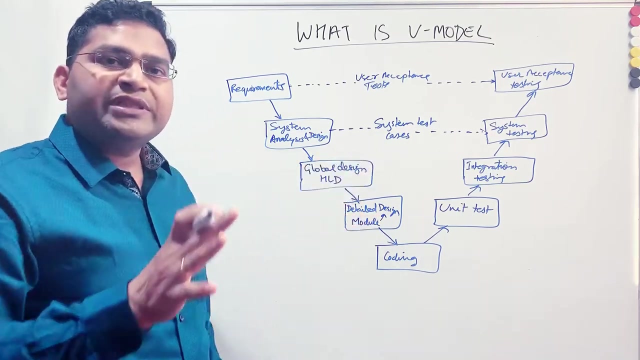 Software development, right. The next phase is basically the global design. When we say global design, so now you have understood about the system test cases. So system test cases will have integration with other systems as well, right, But most of the time, when you talk about the actual core development, it's basically you are developing an application and then that application might integrate with other systems. Okay, so that's what we do in system analysis and design, But the global design is a system test case. 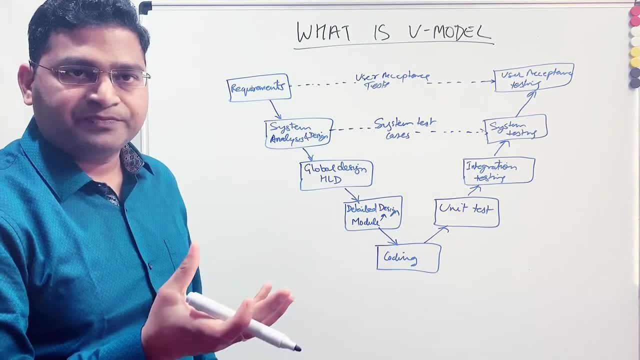 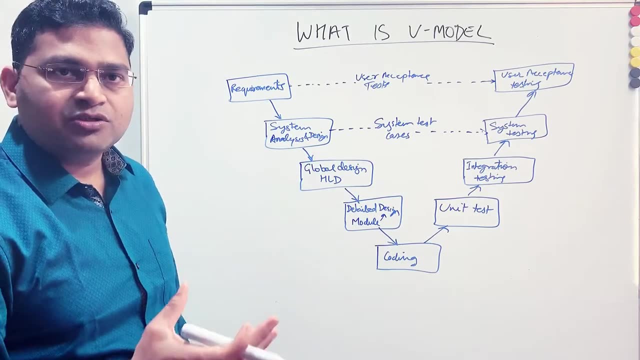 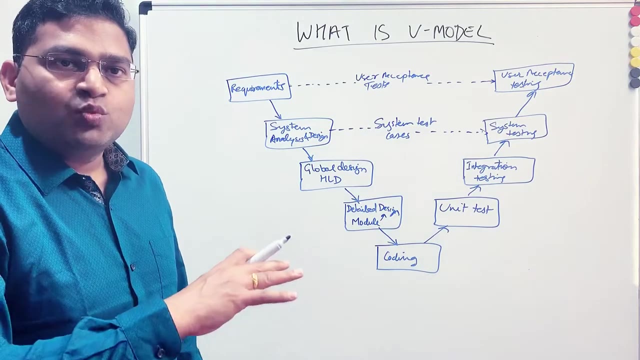 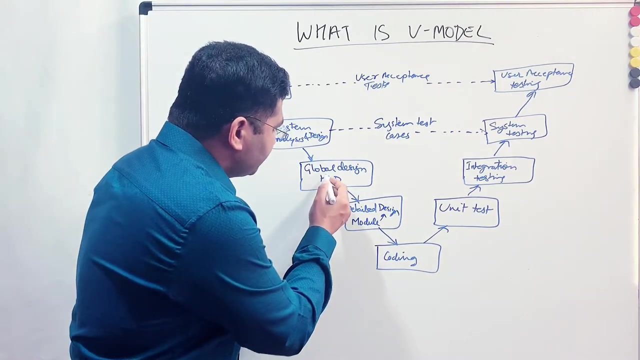 How you will design that core application. Okay, so if I say launching a new card, so what all is required in the core system of the bank to launch a new card or new credit card, So that goes into the global design wherein the tech architects will understand what all is required in the core system to be changed and implemented right. So that is what happens in the high level design And in the system design and analysis: system analysis and design. 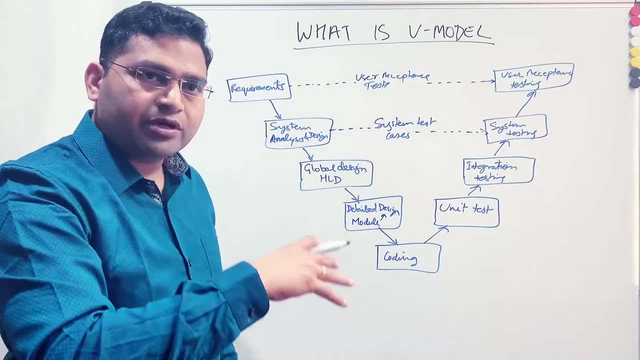 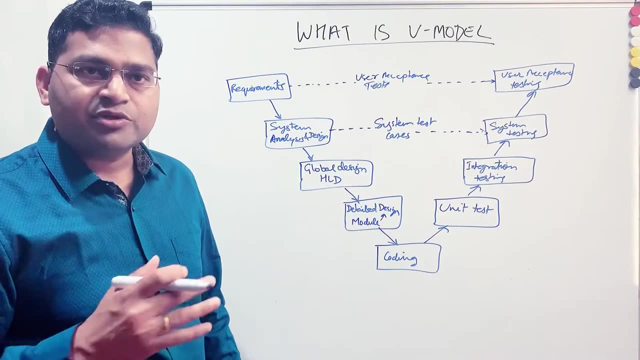 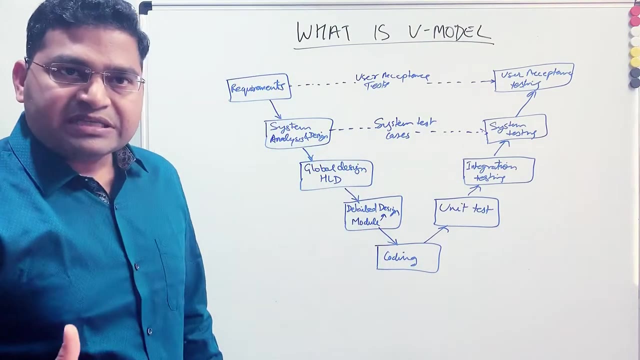 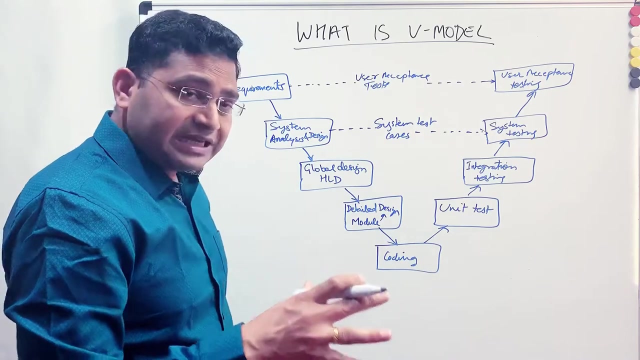 along with that, you know that software or the core design. they think about how that system, the new application they are building, will integrate with third party systems or other systems. That's what happened in system analysis phase. So in the global design phase, once the global design is ready, how the system will be implemented or the software will be implemented in that particular you know that application. then in that phase itself, what testing team does. 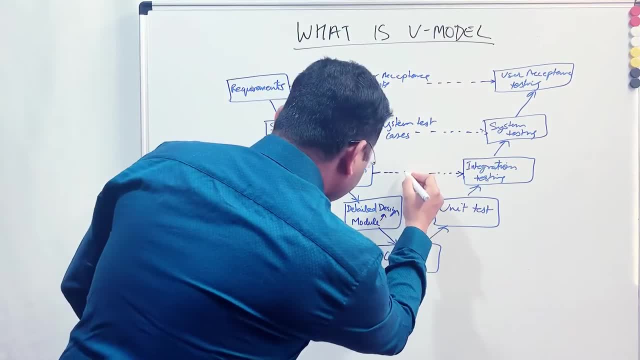 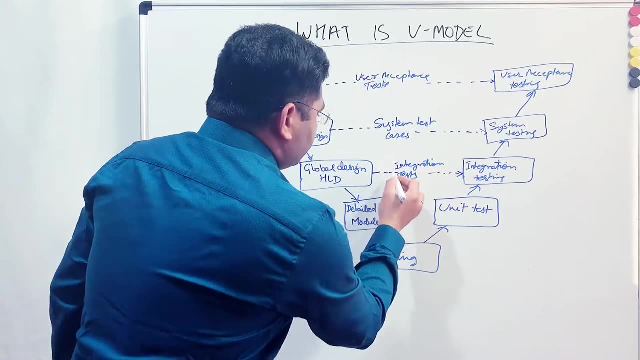 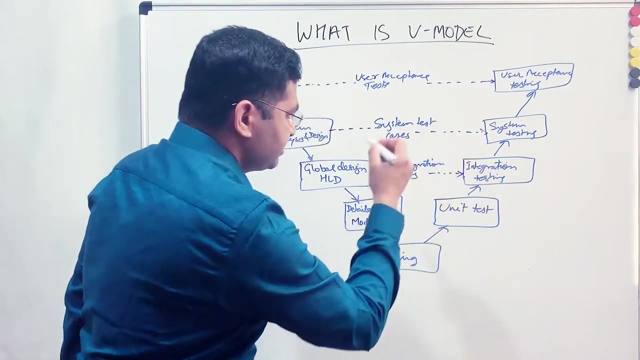 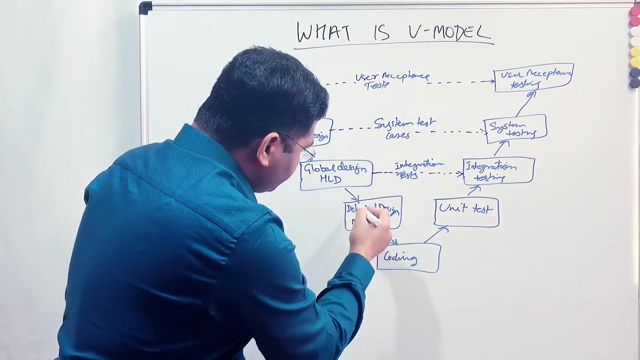 do is they write their integration test cases. right, So they write integration tests. All right. So now, with this phase, the testing is also involved, to write. whenever the design is happening, they write the integration test cases And once the actual code is ready, they'll execute those test cases. Similarly, when it comes to the detail design or the module level design, So when we have the high level design and then the development, 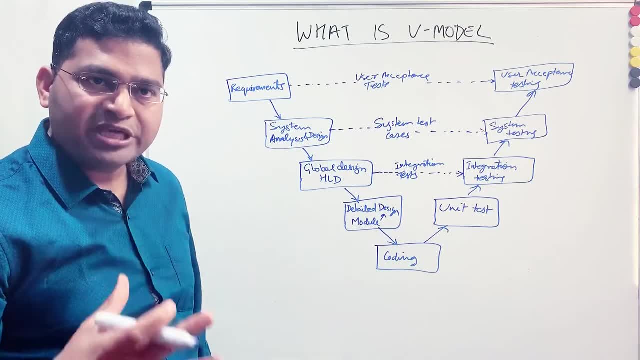 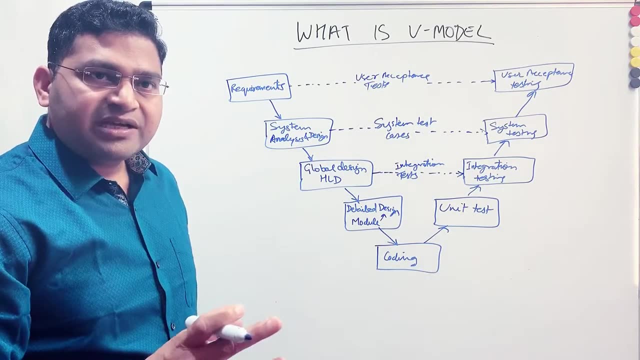 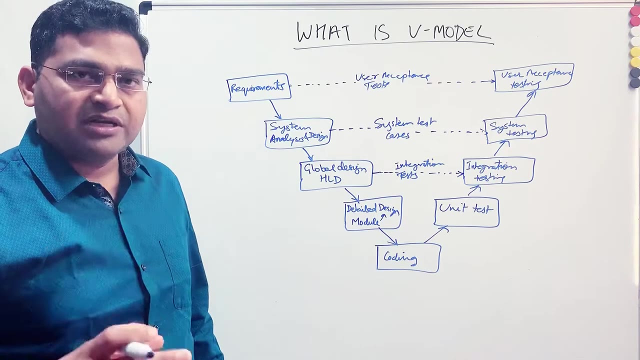 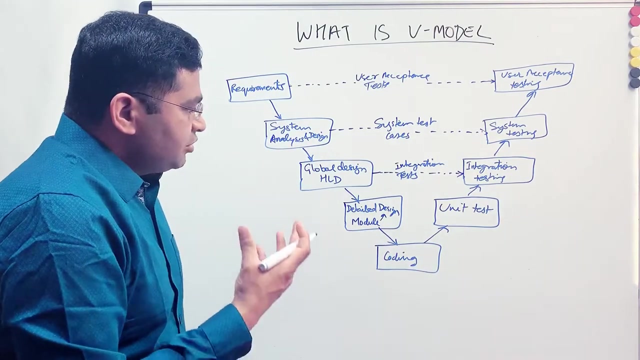 will need to develop small modules to make it, you know, like the overall software, So they won't develop everything all at once. So once the software design is there, they'll break it down into smaller modules and then team will start developing those modules or developers will start developing those modules. That is what happens in the detail design or module level design. So module level design, during the module level design, the testers will go through the module level design and they will 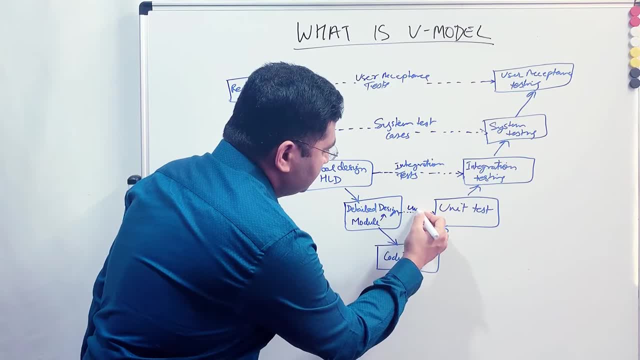 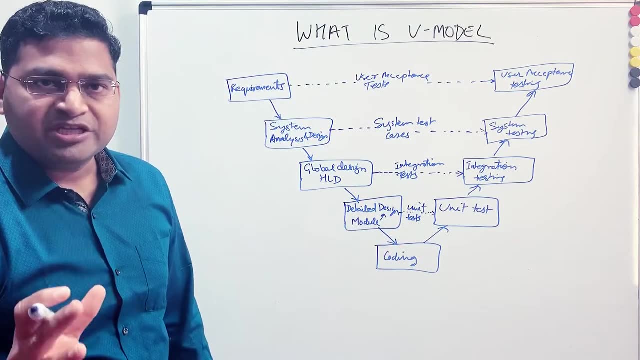 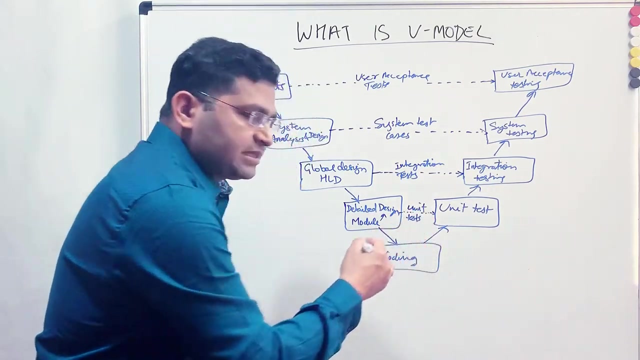 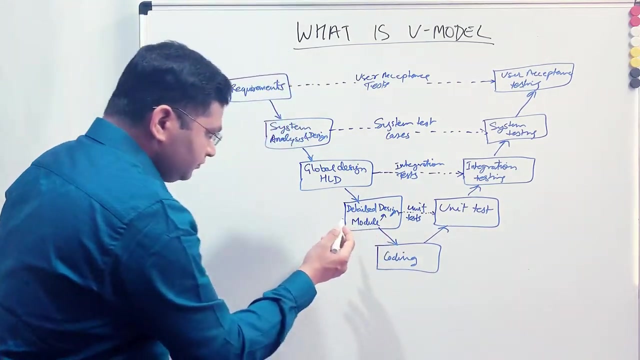 write their unit tests, right? So, unit test. So usually most of the time you'll see, unit tests are written by the development team, But there might be possibility that if you are a white box tester, you might be required to write the unit test cases if you're a tester or white box tester in the team, right? So this is what happens in the detail design or the module design. 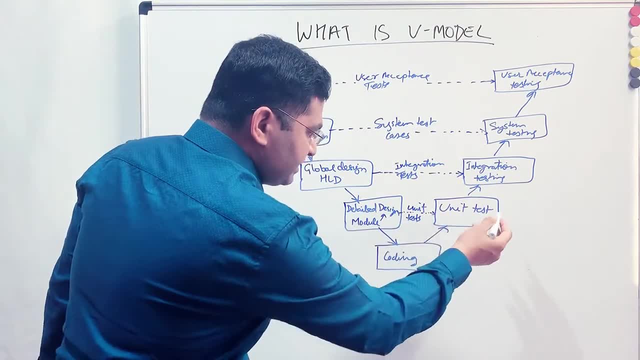 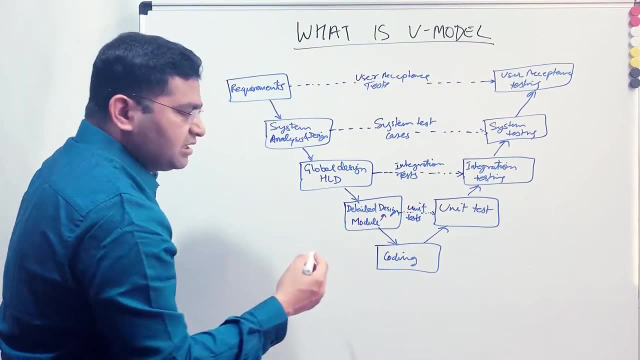 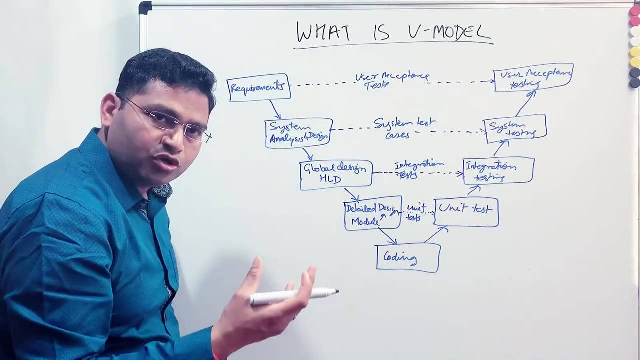 Okay, test cases are being written for the unit test phase. now, once all these design phases are complete, then comes the coding phase. so once the design is ready, or the low level design is ready, then the developers will start coding for those smaller modules. and once those modules are ready, then the 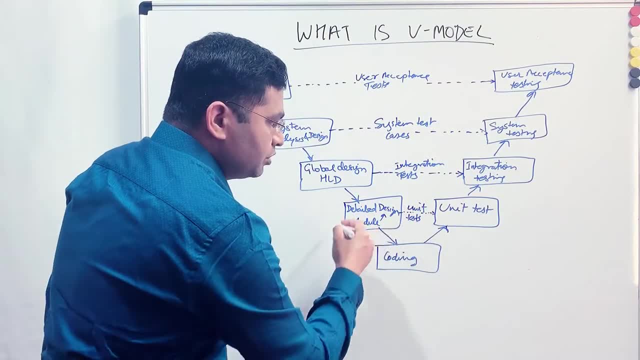 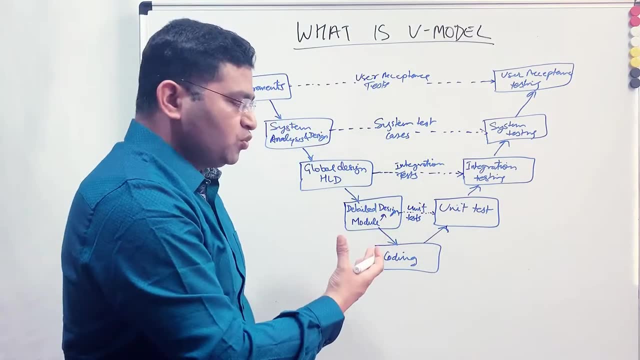 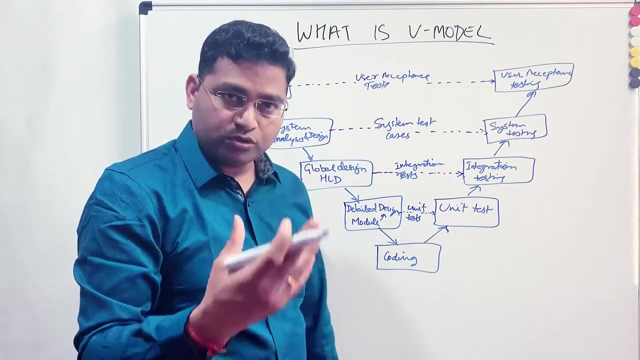 test team because they have already written the test cases. through going through the documentation, they will start testing or doing the unit test right. so once the code is ready, the execution will start. so the actual execution will happen, the application will be launched. so in the unit test case, there will be tools used to do the unit test and if it is one done by developers, 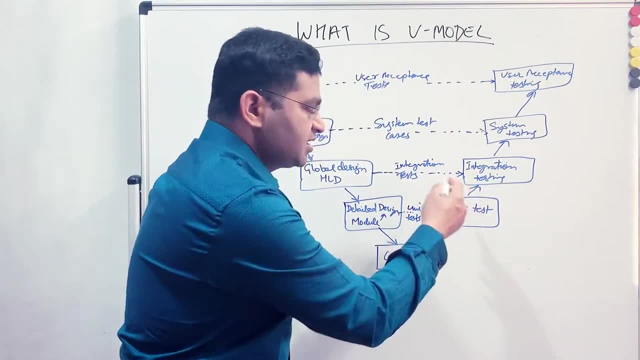 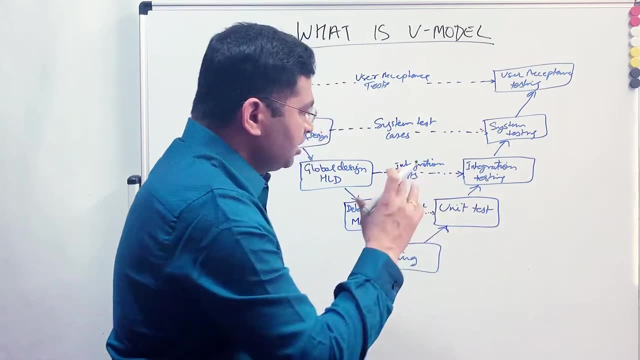 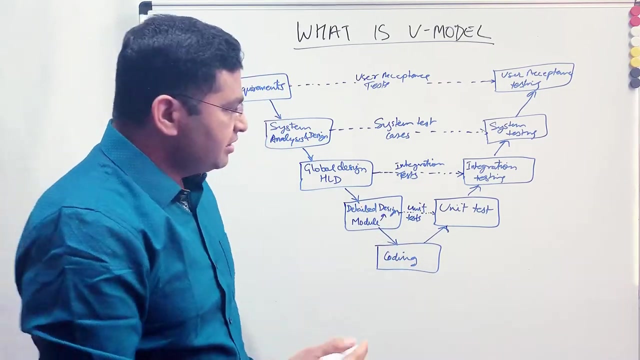 then they'll do it. otherwise, if you're white box tester, you will actually execute the code, whatever developers have coded for those modules, and you will run the unit testing once couple of modules are ready and they are integrated. okay, so couple of modules in the application are ready and they are integrated, say, for example, in the cards. 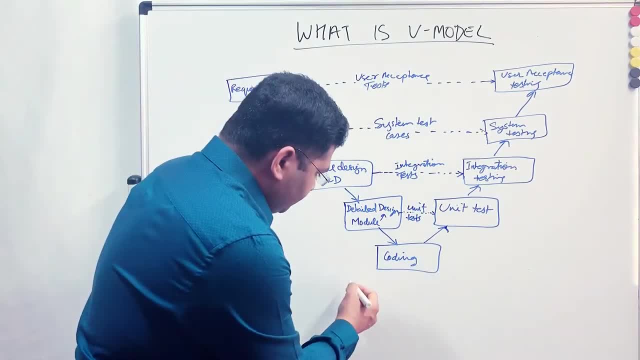 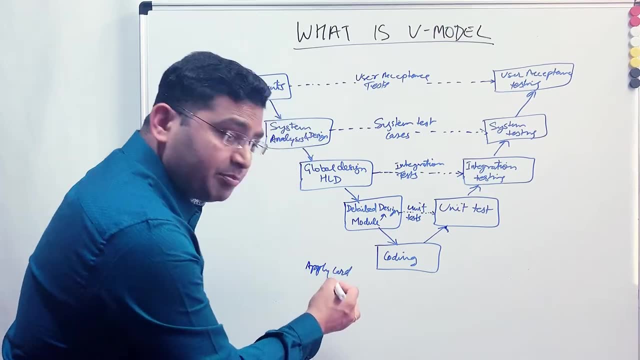 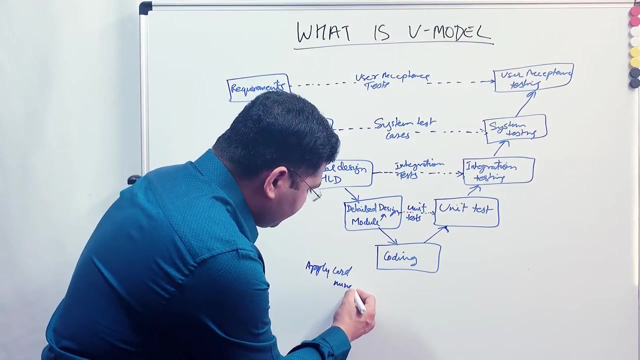 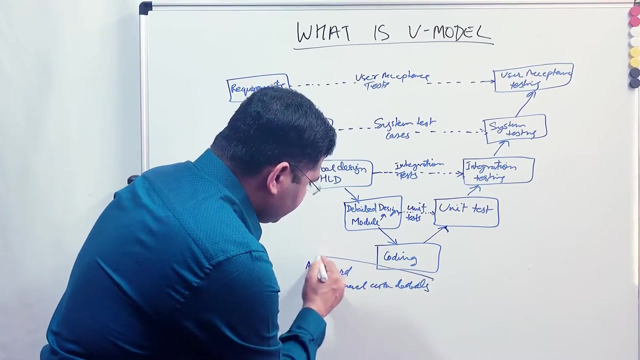 say: we are trying to launch a new card, right, so? so there will be a couple of modules. so apply card, right, so apply card. and even in the apply card there could be, you know, apply card with minimal details. so say, for example, minimal customer details, all right. so say, for example, this is: 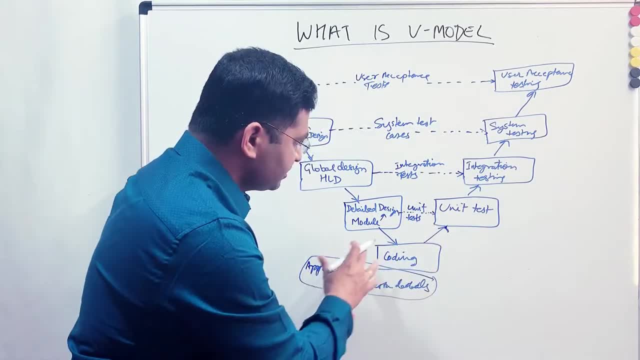 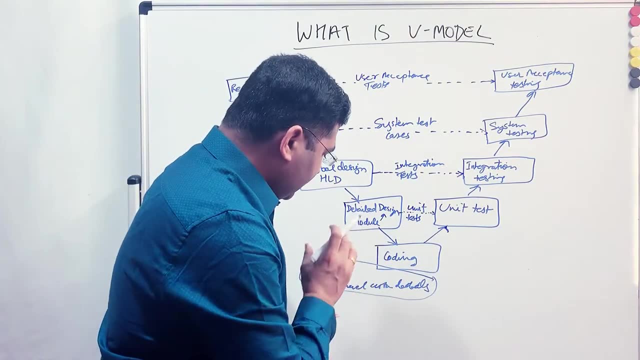 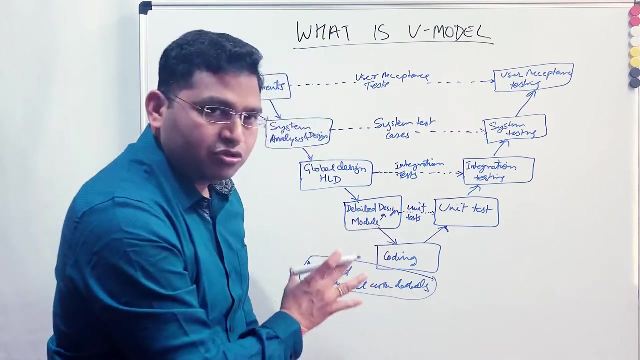 considered as one module. so what you know you will do is, in the unit test, this particular module, you will have a test case which will have the minimal details into that particular module and as part of the unit test they will test this module only okay. similarly, when there are a couple of modules ready. so 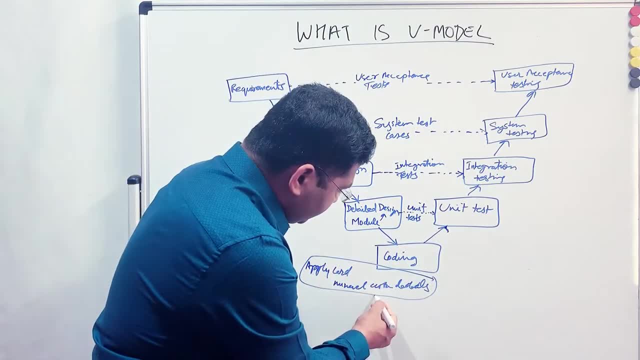 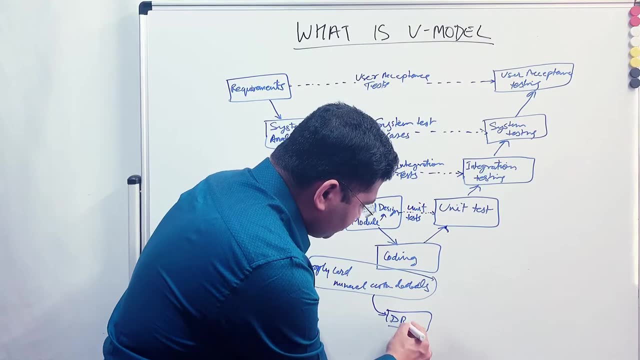 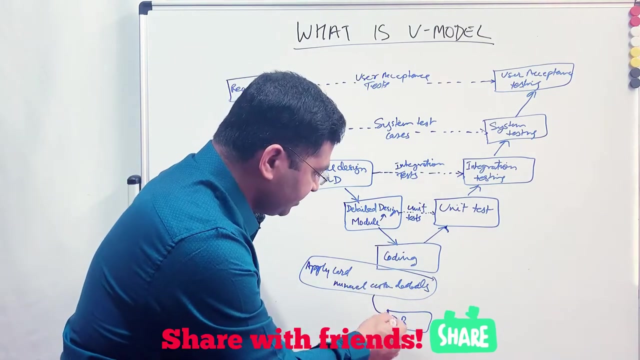 apply card is ready and then this apply card module. once the card is applied, then the card details need to save into the database, right? so this could be another module where there are there is some work that has been done and little bit integration between the front-end and back-end DB has been done. so if 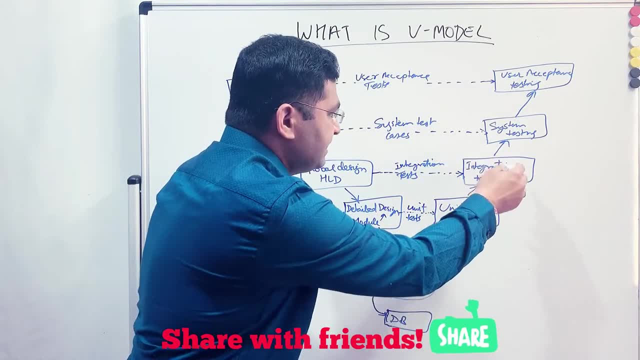 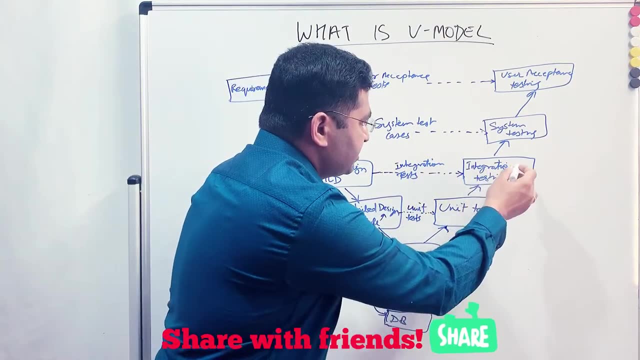 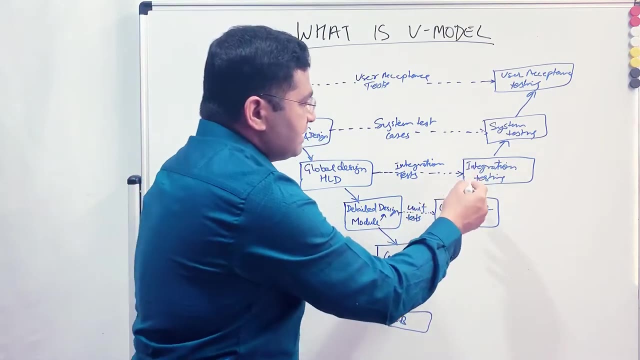 these two modules are integrated. that's what happens in the integration testing. so there are a couple of modules that have been worked upon. if they are integrated, then integration testing is done. okay, so this is what the testing team will do in if couple of modules are integrated, they will start integration testing once all the modules are. 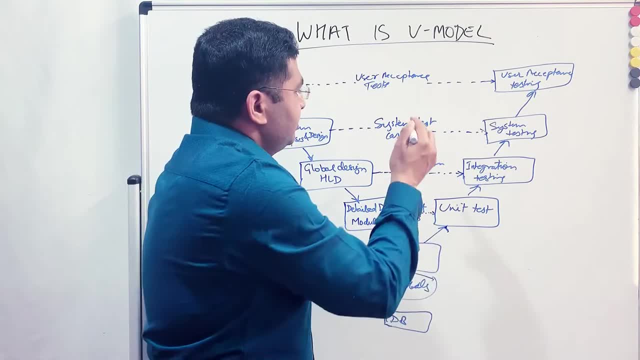 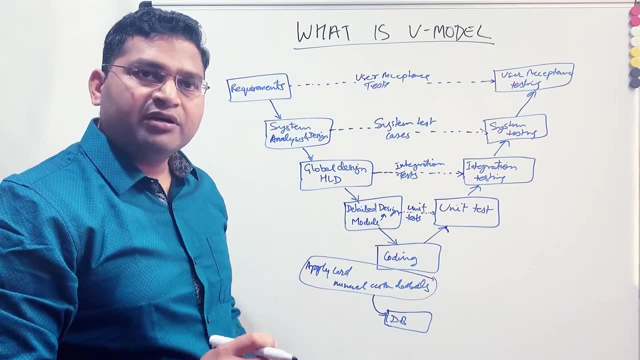 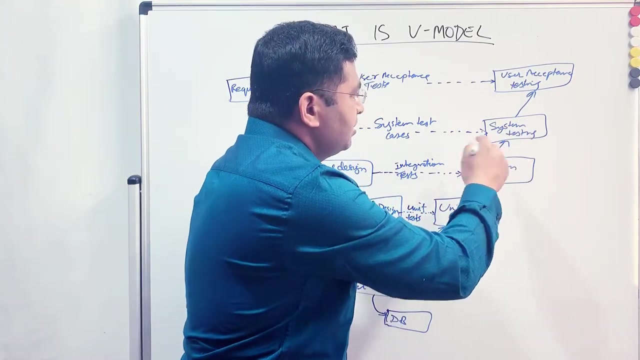 completed, integration testing has been completed, then they'll target at the system level. so the whole software has been developed. now how that software or application is integrated with other third-party systems or other systems, that what happens in the system testing. so the test team, because they have 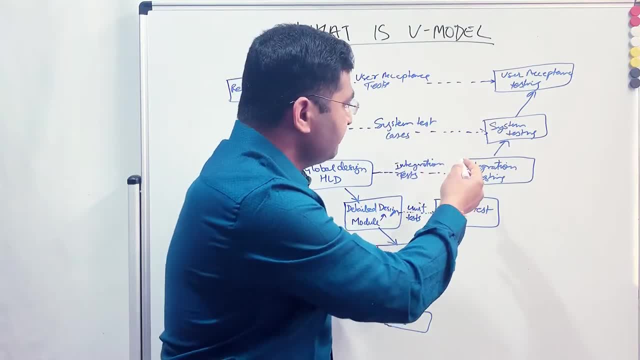 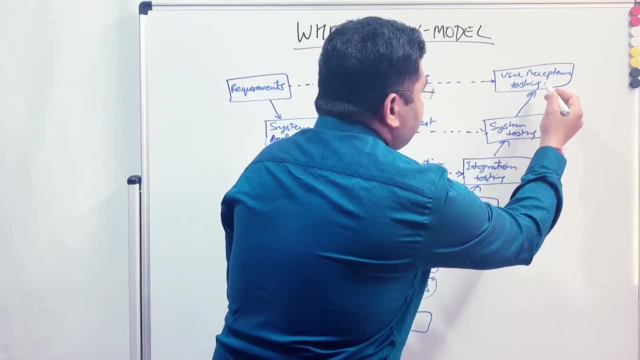 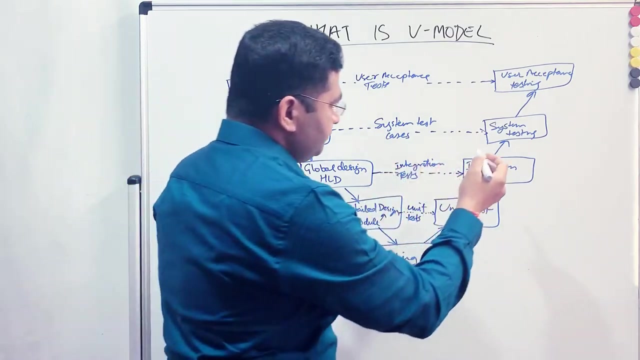 already written, system testing is done, so they will start integration testing test cases. they'll start executing system testing or execute in those test cases. once system testing is passed, then user acceptance testing- which is mostly done by people from the business or, you know, customers in in it, which targets about whatever has been built in the system, whether that is.